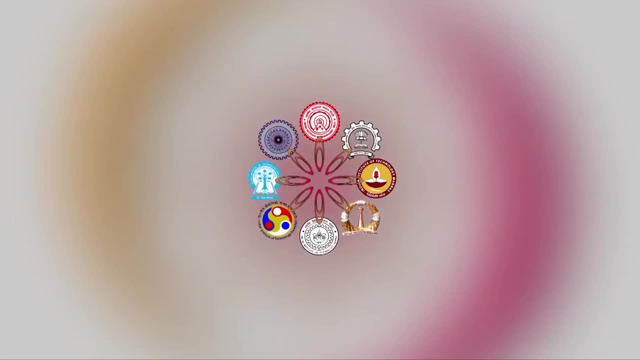 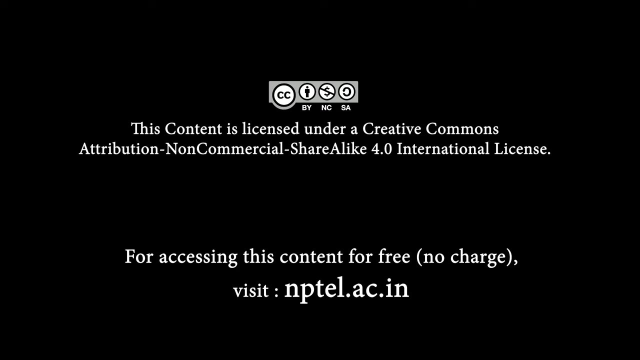 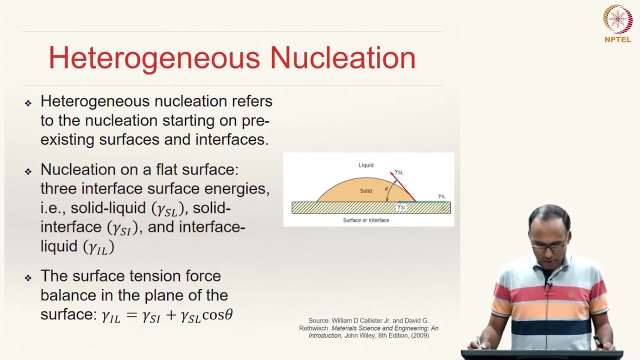 So now let us look at heterogeneous nucleation. Heterogeneous nucleation, as we have already discussed, refers to the nucleation starting on a pre-existing surface and interfaces. There will already be some pre-existing surfaces and there the nucleation happens much faster. 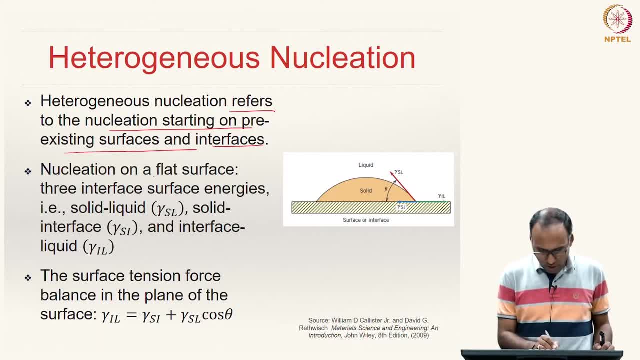 So here we are looking at a nucleation on the case of a flat surface. So when you have a liquid pool and you are having a solid nucleus on a flat surface here, then we can actually see three different interfaces: The interface between solid and liquid, interface between 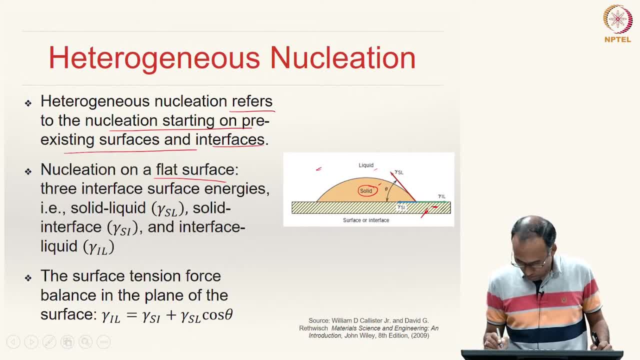 the surface on which- sorry, the interface between the liquid and the surface on which the solidification is happening, the green line- and the interface between the solid and the surface on which solidification is happening, the blue line. So each of these interfaces have certain. 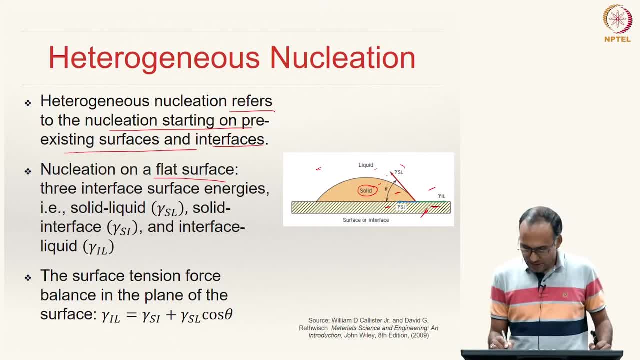 surface energy. So this is what you call gamma SL, the surface energy between solid and liquid interface. I refers to the interface of the solid on which the solidification happening. So gamma IL refers to the surface energy between liquid phase and the surface on which the solidification. 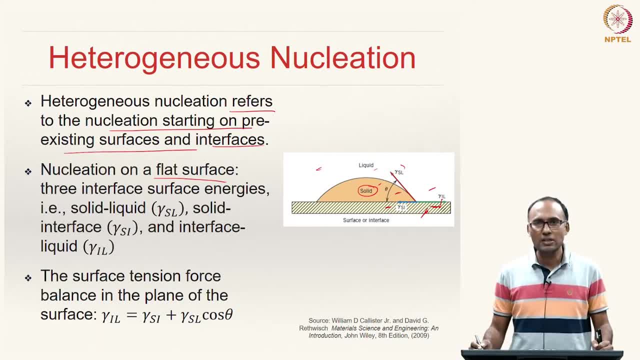 is taking place. and gamma SI indicates the surface energy of the interface between the solid and the solid nucleus and the solid surface on which the nucleation is taking place. So now let us look at the force balance. So let us look at the force balance. 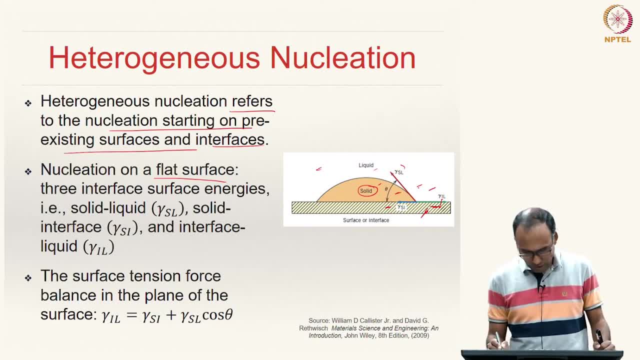 So the force balance here. so the surface tension force in the plane of the surface is given by gamma IL equal to gamma SL, cos theta plus gamma SI right. This is something that one can use in order to write your expressions for delta G or in general. However, we are. 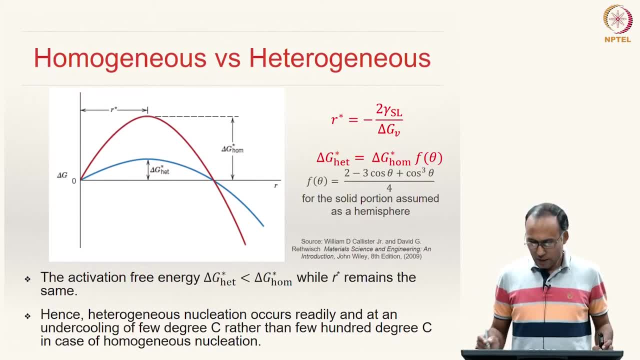 not going through that derivation of how one would obtain the delta G star for heterogeneous nucleation. So if you are interested, I encourage you to go through the text book of Reed Hill on physical metallurgy. There you have a derivation, you have the derivation. 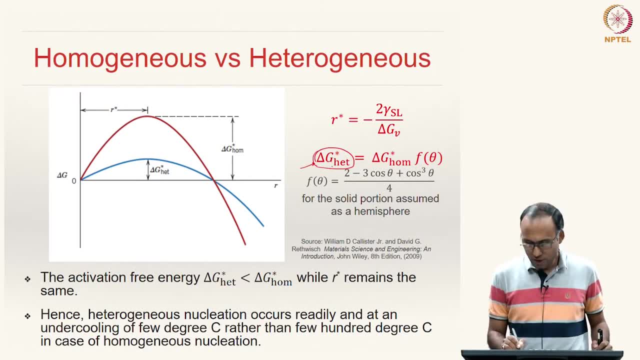 for the for finding the delta G star for heterogeneous nucleation, and in you will see that the heterogeneous nucleations, activation energy for heterogeneous nucleation is related to activation energy for homogeneous nucleation times, some function of theta right. So this theta is what we call wetting angle, as we can we have shown in this figure right. 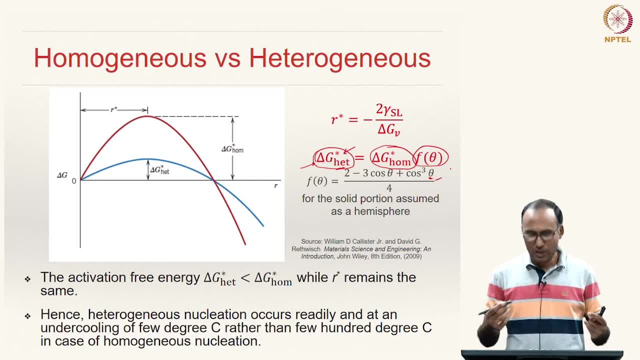 So so f of theta is given by this formula for a spherical particle and you can see that the value will always be less than 1.. So you can see that delta G star heterogeneous. so for the activation energy for heterogeneous nucleation is out Normally. delta G, 0 star. 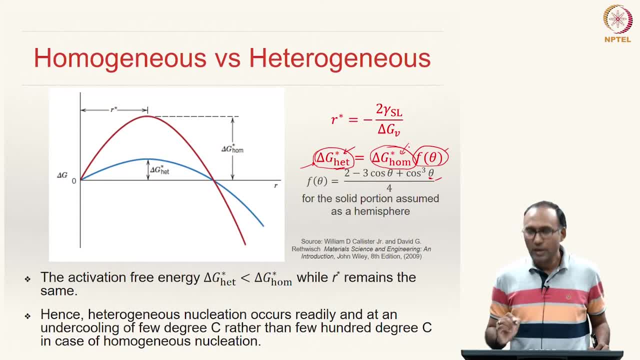 Now thehopунк miles per second. I am not takąplating it now. bése met andi bomni. not impossible is known. There are other types, which is white. So if you have number p, there always going to be less than the activation energy required for homogeneous nucleation. 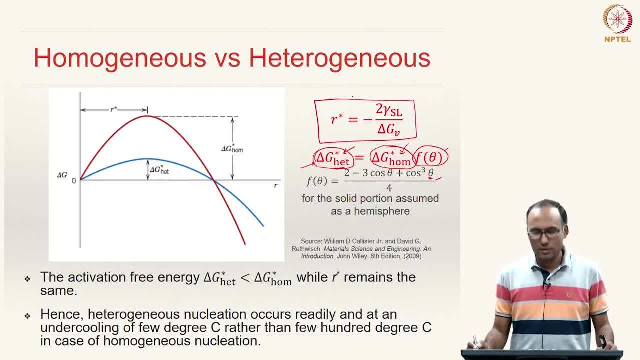 However, the r star remains same. So this is gamma between solid and liquid interface. So the solid and liquid interface. solid means for nucleus, solid nucleus and liquid interface. gamma is going to be same whether you are having homogeneous or heterogeneous. the surface, energy is, surface is going to be the same and hence the r star value is not going to. 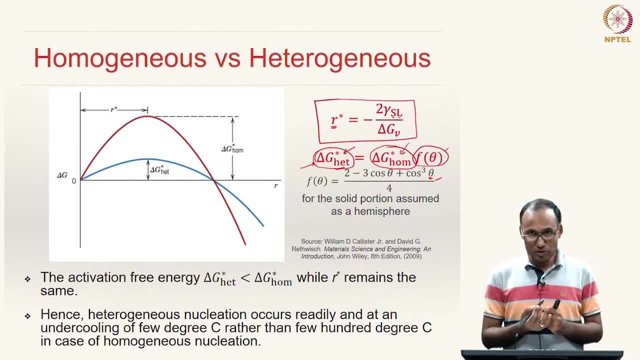 change. ok, So the for homogeneous and heterogeneous nucleation for the same critical radius. you see that you need much lower activation free energy for heterogeneous nucleation compared to homogeneous nucleation. that is why it is much easier to have heterogeneous nucleation, So heterogeneous nucleation happens much more readily than homogeneous nucleation. 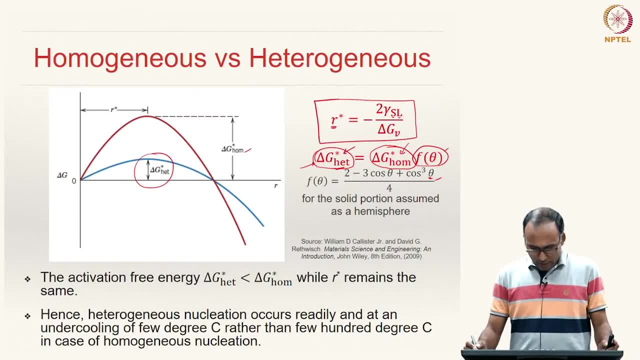 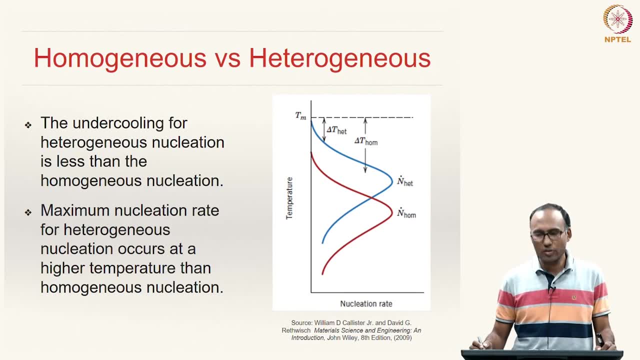 So all right, and if you see the degree of under cooling required for heterogeneous nucleation and homogeneous nucleation, this graph clearly shows that the n dot for homogeneous nucleation curve is little down from heterogeneous nucleation. So this is what we have looked at, the red. 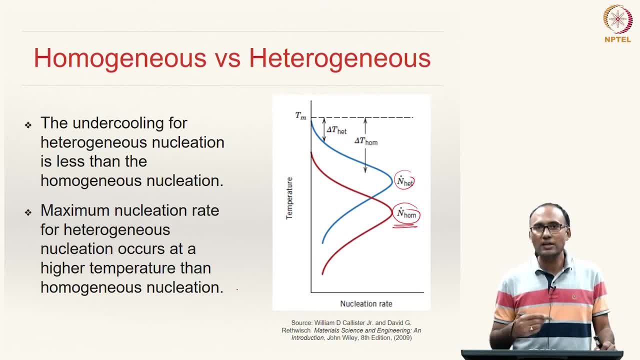 curve before the heterogeneous nucleation turns out that the degree of under cooling required for heterogeneous nucleation is only few degrees Celsius, not few hundreds of degree, few hundred degrees Celsius, like homogeneous nucleation. that means the heterogeneous nucleation can actually happen at much higher temperature than homogeneous nucleation right and as a result, the curve shifts upwards. all right, 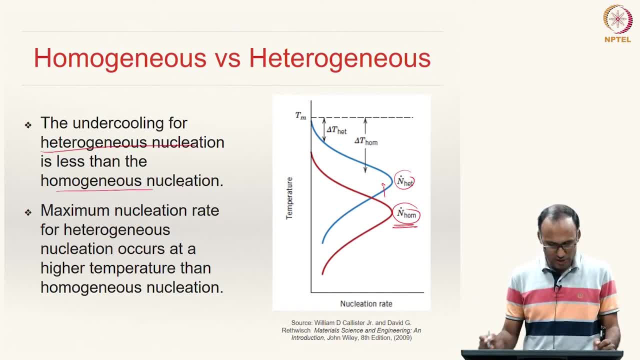 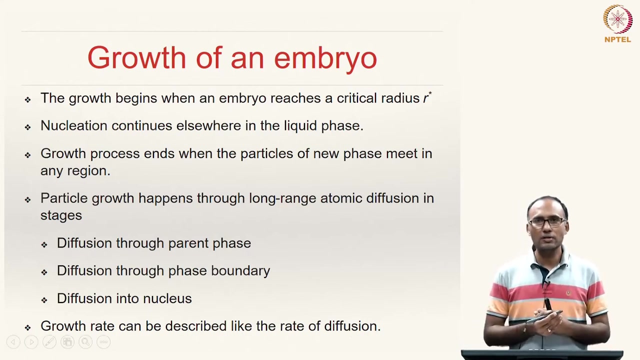 So the under cooling for heterogeneous nucleation is less than the homogeneous nucleation and the maximum nucleation rate n dot for heterogeneous nucleation occurs at higher temperature than for homogeneous nucleation rate. alright, So having looked at now under having understood the concept of nucleation and the two different types of nucleation- homogeneous nucleation- 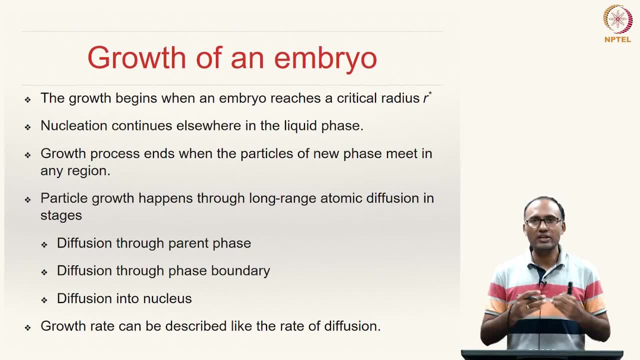 and heterogeneous nucleation and the nucleation rate. that means rate at which the number of nuclei are forming in these two different types of nucleations. Now, once you have certain nuclei formed and the next step is growth of this nuclei. right, that means more and 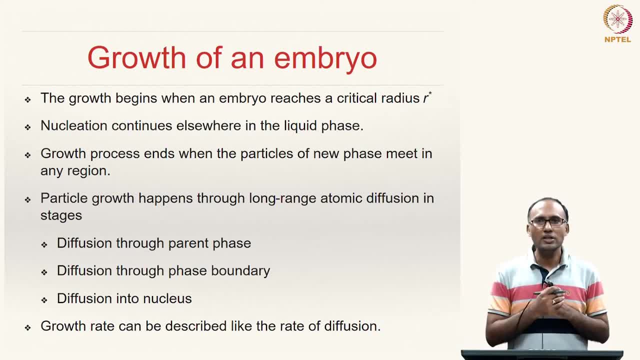 more liquid has to come through diffusion and join the solid phase in order to increase the size of the solid phase. So, as we have discussed, the growth begins when embryo reaches a critical radius, r star. So below that radius it again dissolves, but only when the nuclei 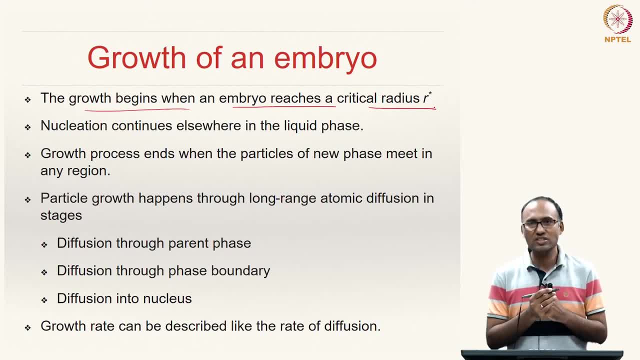 reaches this radius r star. only embryo reaches this radius r star. that is when it is called nucleus, and it is, it can, it is ready for growth. So once you have a certain nucleus formed a one place in the liquid solution, while this is growing there, it is still possible that 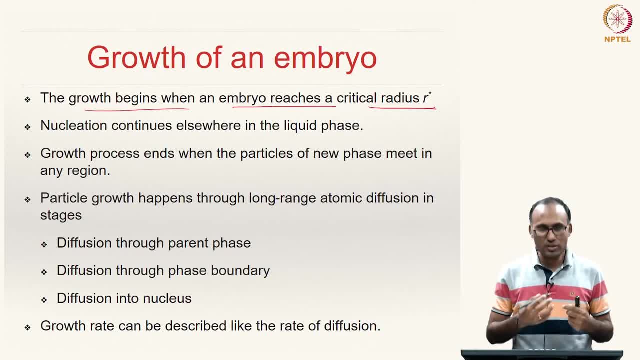 the nuclei can still continue to form at other locations, right? So they can happen simultaneously. So the nucleation continues elsewhere in the liquid phase and, however, this growth process hence. So suppose, if you have one nucleus here, another nucleus here and then 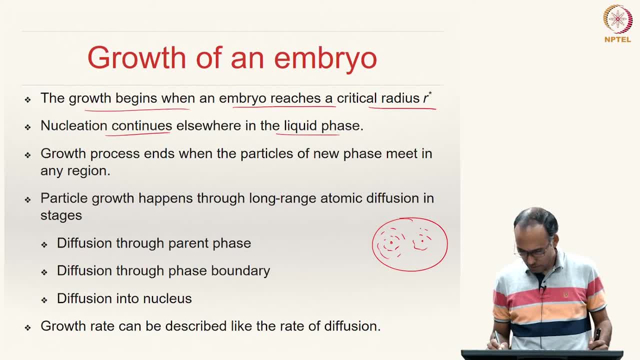 this guy is growing. this guy is growing and then the moment these two guys hit, that means when these two nuclei which are growing this growth process, hence when the particles of new phase meet in any region. So if you are here, then the new, the growth here stops and 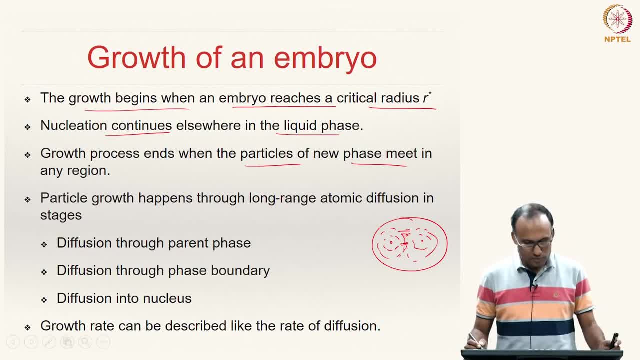 then it continues in this region and so on, As we can see that the particle growth happens through long range atomic diffusion in different stages. So what are these long range atomic diffusion? you can have the diffusion through the parent phase. FINAL FASHION OF CLIENT 1имиher ND eenabe compared to 60 t flop. parent phase measurements of the. 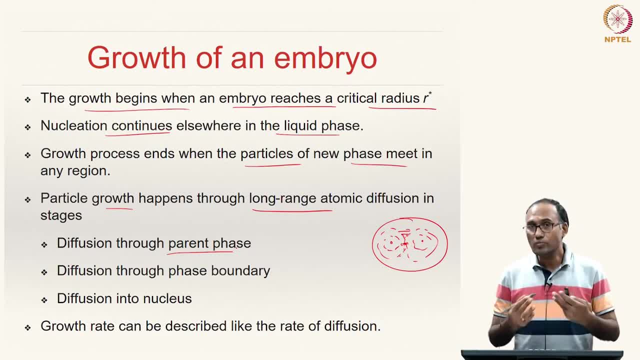 coespère Di-o-edifl. parent phase is the, per instance, liquid phase and diffusion through the phase boundary: from the liquid phase to the solid phase, through the phase boundary. it has to cross the phase boundary and within the solid phase again there has to be some diffusion. So diffusion. 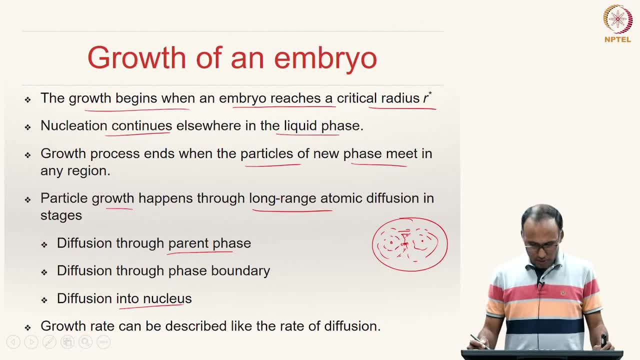 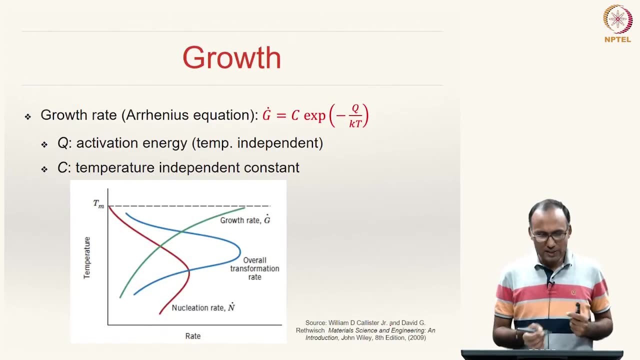 into the nucleus from there right. So the growth rate can be described like the rate of diffusion, which is pretty similar because the growth is a diffusion process. So the growth rate can be described by Arrhenius type of equation, as shown here. g dot is equal. 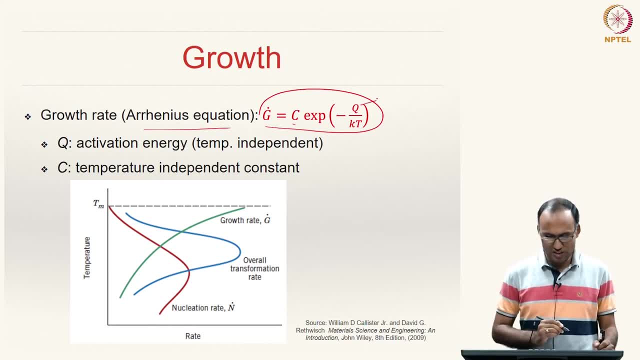 to c times e power minus q by k t, where q is your activation energy, which is temperature independent, and c is our temperature independent constant right. So now, if you would plot the growth rate g dot, it looks like this green curve. So this is our growth rate. as you are at higher temperature, you know that the diffusion is. 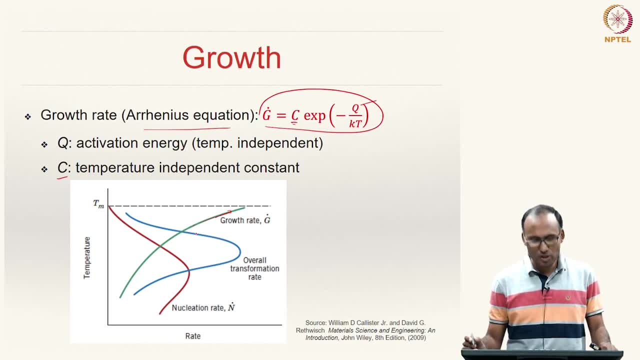 faster at higher temperature and, as a result, you will have higher growth rate. at low temperatures, the growth rate is low and this is our. the red curve is only a part of the nucleation rate. this is there is also somewhere here, but we have not shown that this is our nucleation. 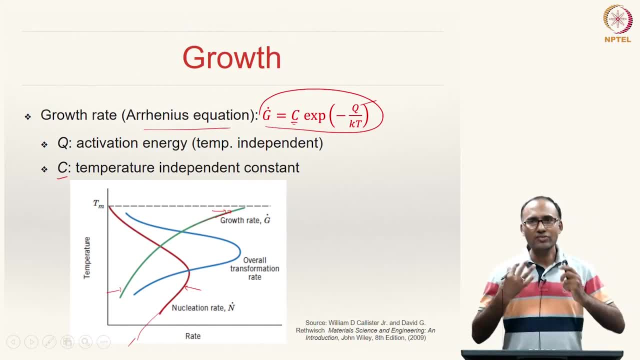 rate. So now you have certain nucleation rate and some A growth rate, and now you can actually plot the overall transformation rate using these two quantities and the overall transformation rate looks something like this: So the overall transformation rate increases as you reduce the temperature and reaches a maximum value. 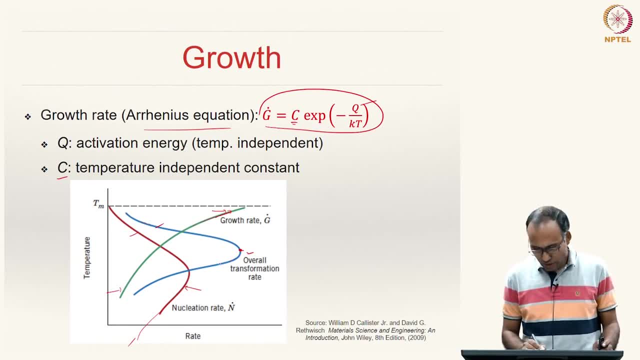 and then it starts decreasing again, because at this point your, although your nucleation rate is increasing, but your diffusion is decreasing significantly and hence your overall transformation rate reduces. At the top we have very high nucleation rate and, sorry, low nucleation rate, So that means very few nuclei. number of stable nuclei will be less at high. 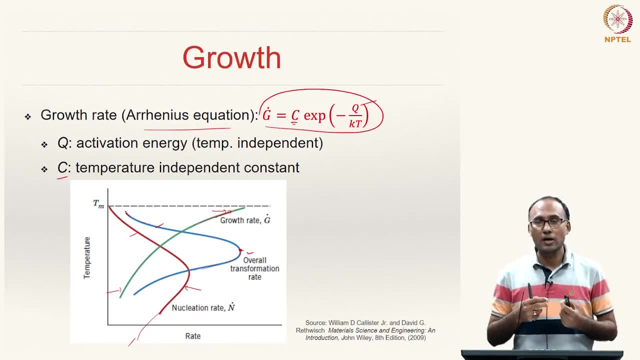 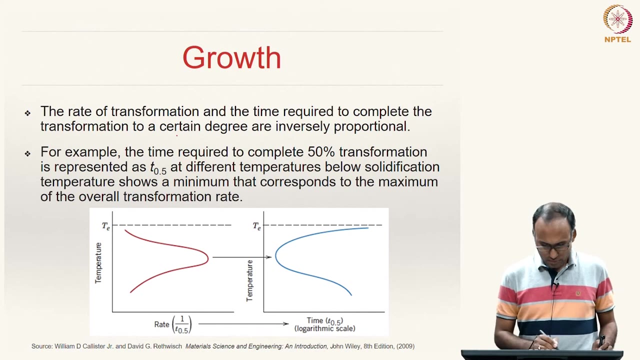 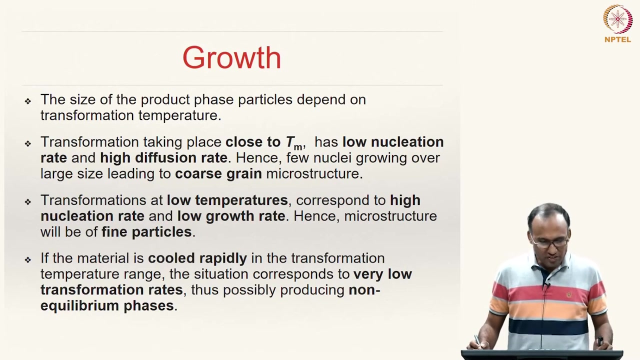 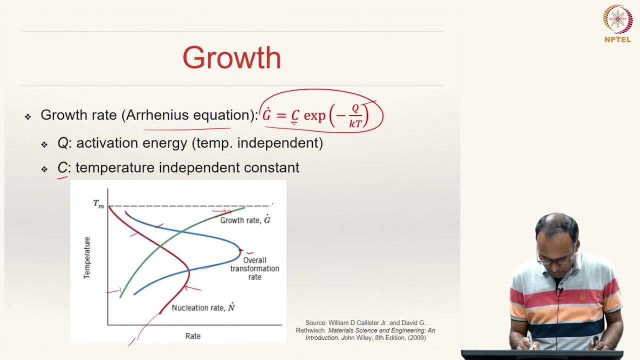 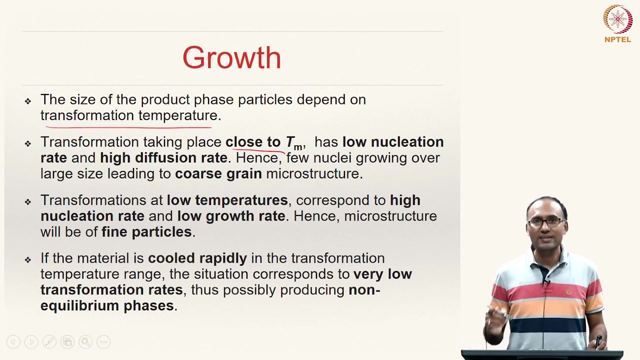 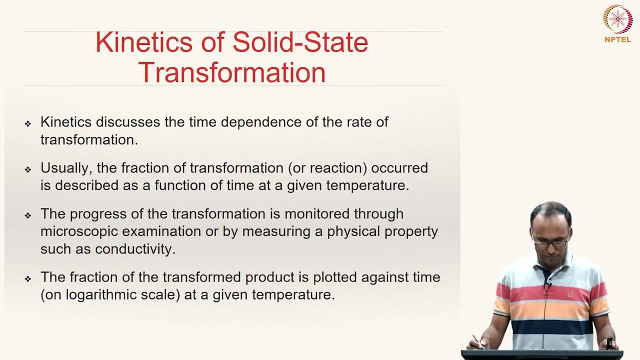 temperature, but the growth rate is large. that means the rate at which the particle grows is very large. here that means the diffusion is. diffusion can happen over long distances at high temperatures. So this is what fraction of the material has been transformed, and then the fraction. 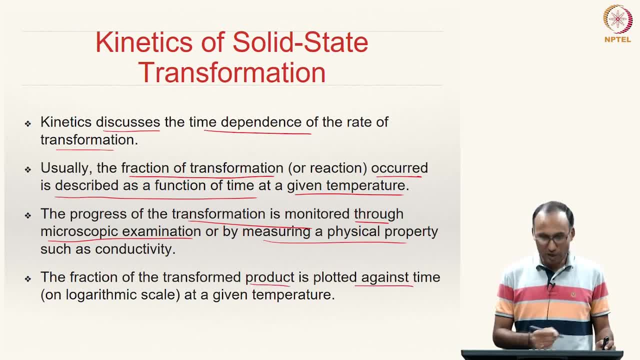 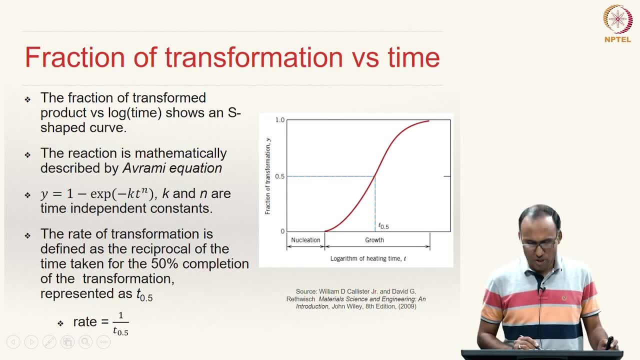 of the transformed product is plotted against time on a logarithmic scale at a given temperature, right? So now let us look at the fraction of transformation as a function of time, as you know that it takes some sufficiently long time, depending upon the temperature at which. 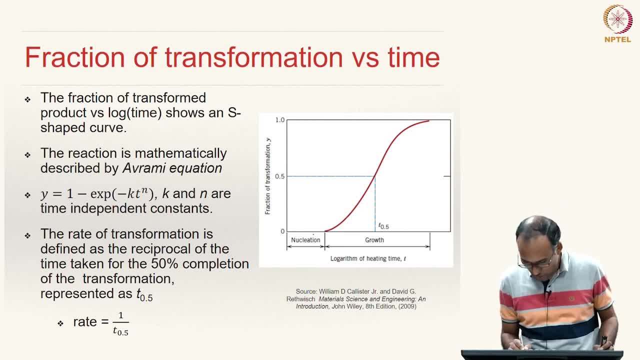 you are actually doing this transformation. It takes some time for nucleation, So initial time, up to certain time, there will not be any growth. So this is what fraction of the material has been transformed, and then the fraction of the transformed product is plotted. 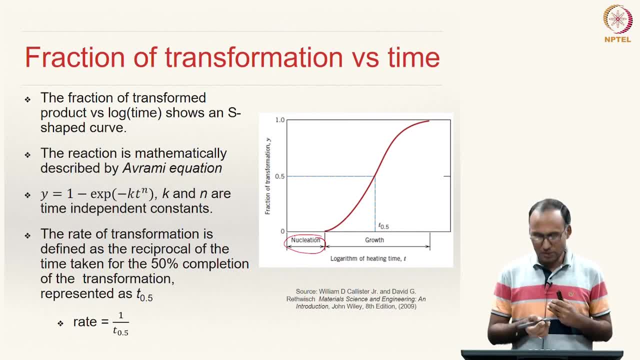 against the growth because the system is nucleating particles or nuclei and after nucleation is finished, that is when the growth begins, right. So the fraction of the transformed product. so on the y axis we are showing fraction of the transformed product here up to growth. 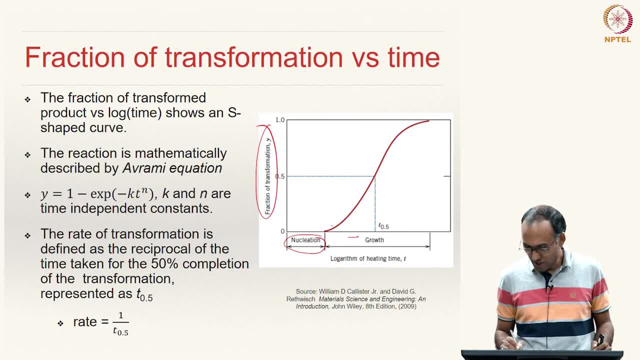 beginning there is no transformation and as you are increasing the temperature, from that stage the fraction of the transformation increases asymptotically to 1 right. So this state is our growth state. So in this equation, the this curve looks like an S shaped curve, which can be mathematically 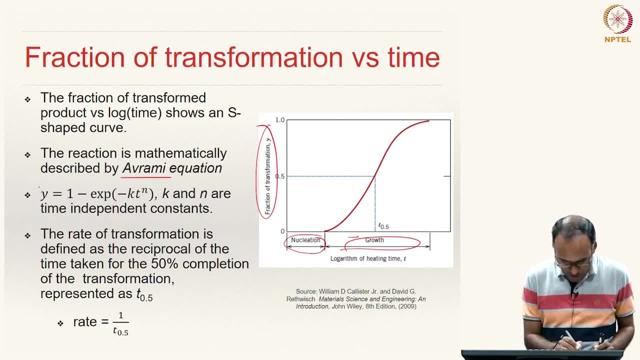 described by something called Avrami equation, as given by this relation: y equal to 1 minus e, power minus k, T power n, where T is the time, k is k and n are time independent constants which depend on temperature at which this transformation is taking place. So here the 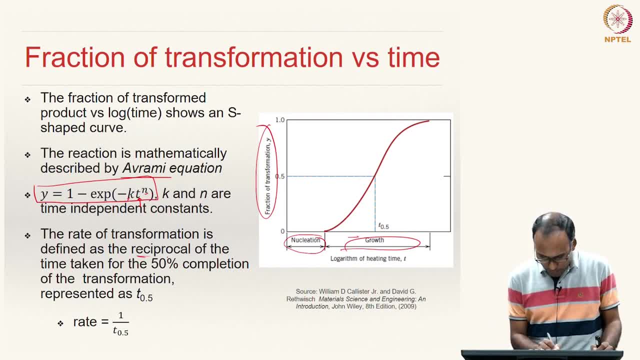 rate of transformation is defined as the reciprocal, The reciprocal of the time taken for 50 percent completion of the transformation, represented by T 0.5.. So that means if you are talking about rate of transformation, you are saying that the it is defined as the reciprocal of the time taken for 50 percent completion of. 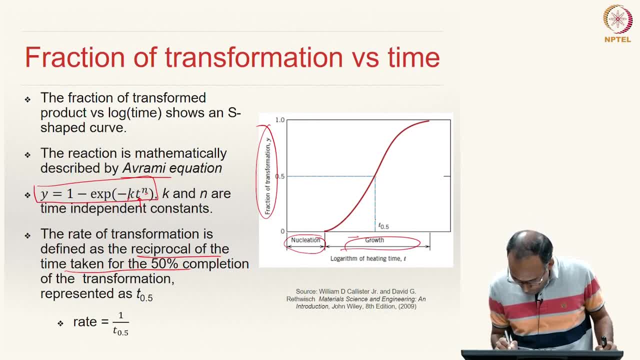 the transformation. So if you are, you can see that here. this is the time taken for 50 percent completion of the transformation. then the rate is described as 1 over T 0.5. all right, So with that we have understood how a new 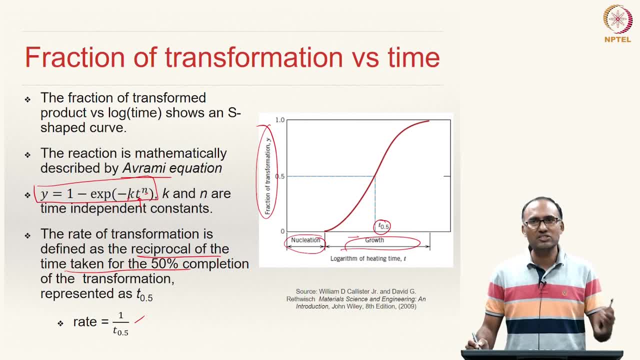 experience can be achieved by discussing the mechanismsome of describes of the aircraft and Is our. And then we have discussed the difference between heterogeneous nucleation and homogeneous nucleation, And we have looked at the fact that the heterogeneous nucleation has lower. 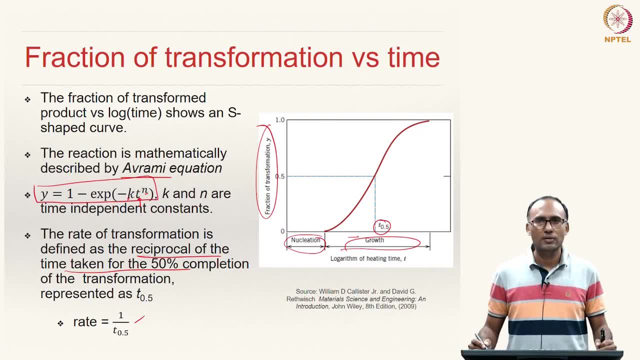 reactivation energy compared to homogeneous nucleation. Then we have discussed the concept of nucleation rate and we have shown that the nucleation rate is going to have a maximum at a certain temperature And the heterogeneous nucleation rate occurs at a higher temperature. 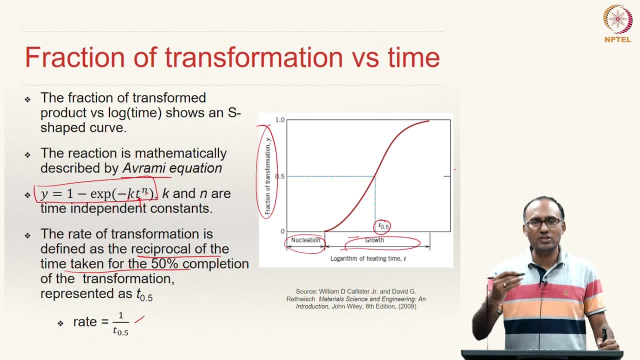 maximum value of heterogeneous nucleation rate occurs at a higher temperature compared to homogeneous nucleation, And the degree of under cooling required for heterogeneous nucleation is less than the degree of under cooling required for homogeneous nucleation. And then we have discussed the growth process and how the growth process is described by. 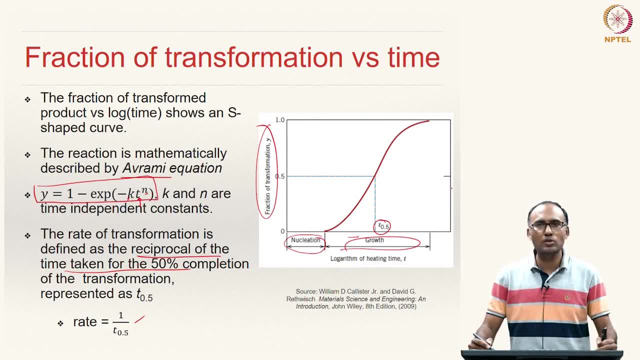 a diffusion like phenomena, And then we have shown that the growth is higher at high temperatures and reduces at low temperatures, because at low temperatures the diffusion is low And the overall transformation rate also is shown to have a maximum at certain temperature below the T m. And then we have also looked at the transformation rate as a function of time. 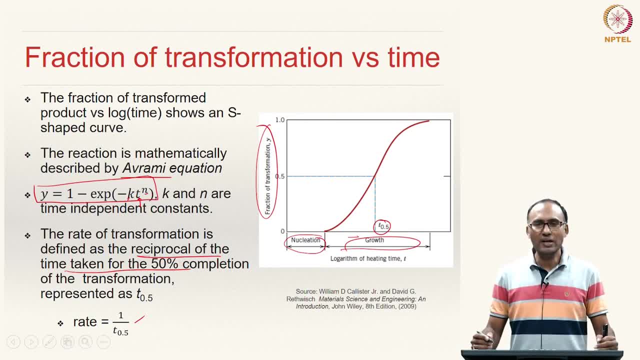 for different, at different temperatures. And finally, we looked at the fraction of transformation as a function of time. So, as a function of time, how much amount of material has been transformed from parent phase to product phase, and that is described by Avrami. 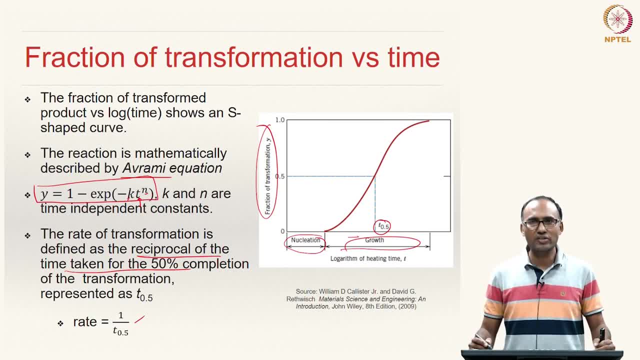 equation wherein the fraction of transformation, when plotted against time, looks like a S shaped curve, as shown here In the next class we will use this knowledge in order to understand the important concept called isothermal transformation and we will diagrams in the, particularly for steels. Thank you very much.